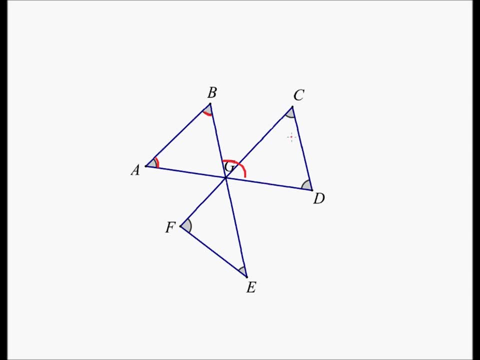 Using a very similar argument, I can say: this angle in green plus this angle in green should equal this angle in green. Why, If this angle is A, these two angles should add up to 180 minus A And this angle alone should be 180 minus A. So they better be equal. 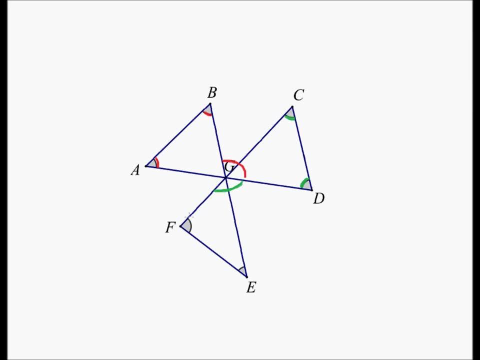 Okay, Using a very similar argument, I can say: this angle plus this angle should add up to this angle. Why? Exact same argument: If this angle is C, these two angles, this angle and this angle, should add up to 180 minus C. 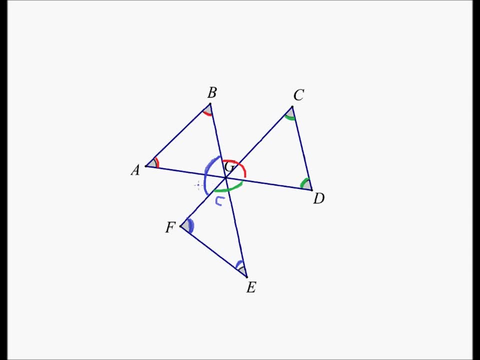 And this angle should also be 180 minus C. Therefore, these two blue angles should add up to this big blue angle here. What do we know about these three angles? Let's use light purple to circle this. What about these three angles back here? The big red angle, the big green. 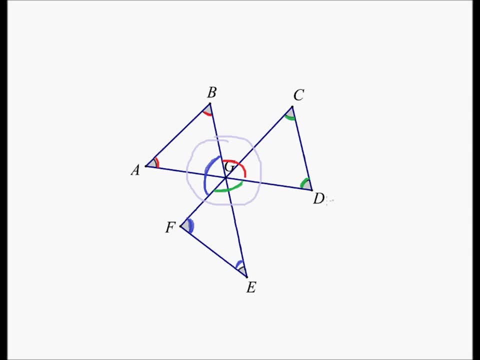 angle, the big blue angle. Well, these three angles should add up to 360, 360 degrees. So the sum of these three angles should be 360 degrees. Why? Because they are all around a point. Now, based on that, we can conclude: 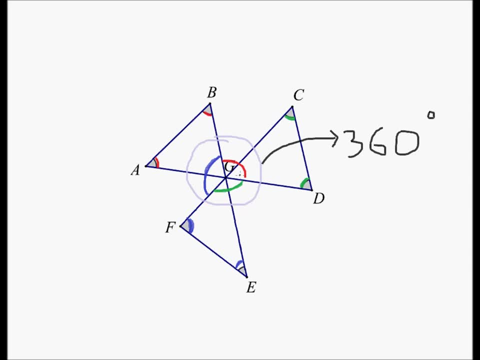 these two red angles, this one, this one plus these two green angles, this one and this one plus these two blue angles, this one and this one should also add up to 360.. So that's the explanation why angle A plus angle B plus angle C plus angle D. 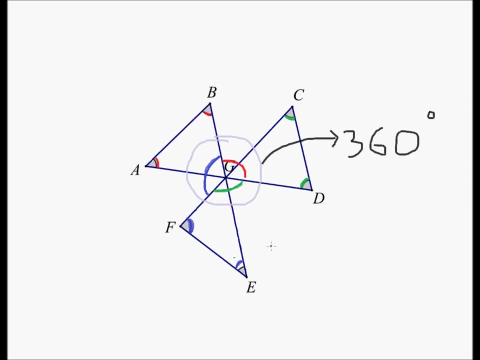 plus angle E, plus angle F should equal 360..